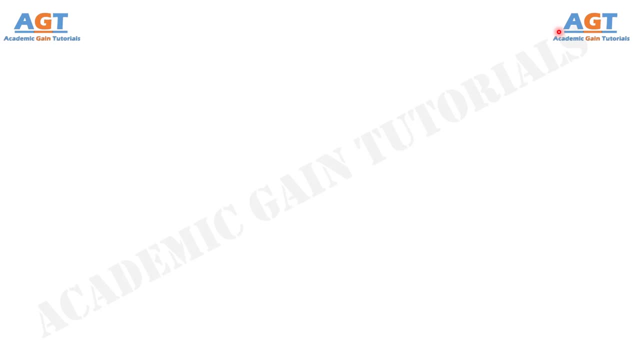 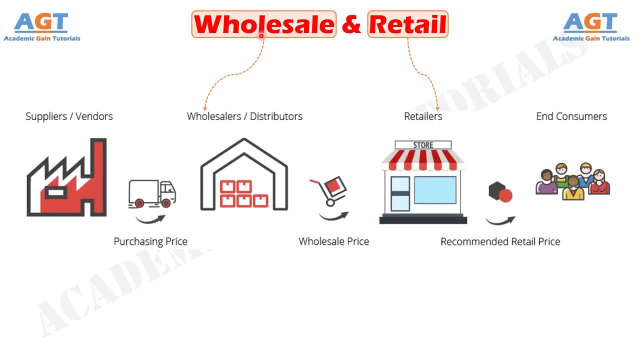 Welcome to Academic Game Tutorials. In this video we will look into the differences between wholesale and retail. The word wholesale simply means selling in bulk quantities and retail stands for selling merchandise in small quantities. Wholesale and retail are two distribution arrangement that constitutes a major part of the supply chain. 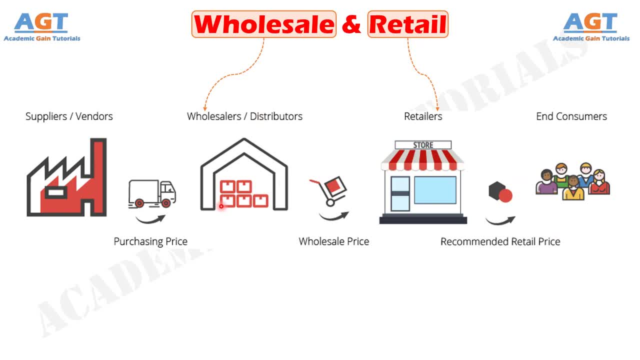 While a wholesaler sells goods to the businesses as they purchase goods to sell it further, on the other hand, a retailer targets final consumer and sells goods to them. So let's look into the basic differences between wholesale and retail in a tabular form. 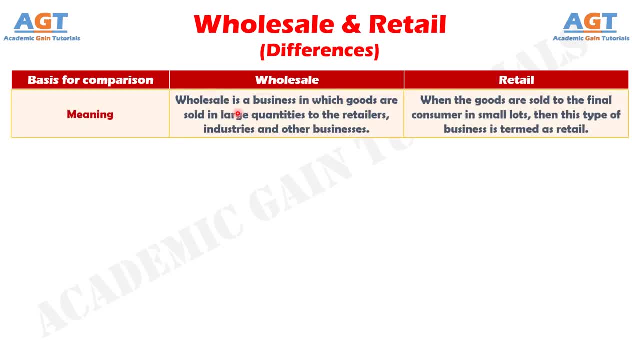 Difference number 1. Wholesale is a business in which goods are sold in large quantities to the retailers, industries and other businesses, Whereas when the goods are sold to the final consumer in small lots, then this type of business is termed as retail. 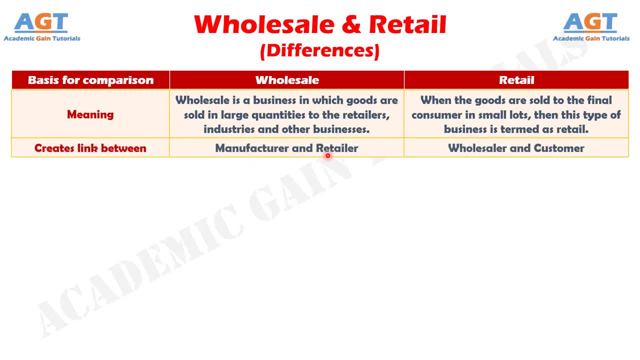 Number 2. Wholesale creates a link between the manufacturer and retailer, whereas retail creates a link between wholesaler and customer. Number 3. There are wide differences between wholesale and retail price of a particular commodity, That is, the wholesale price is always less than the retail one. 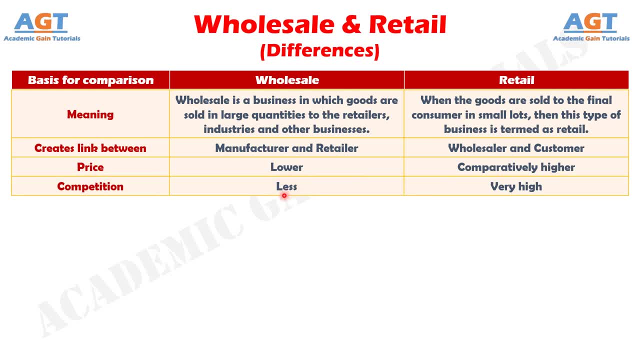 Number 4. Competition is less in wholesale segment, whereas competition is very high in retail segment. Number 5. Volume of transaction large in wholesale, whereas volume of transaction is small in retail. Number 6. In wholesale business the capital requirement is higher than in retail business. 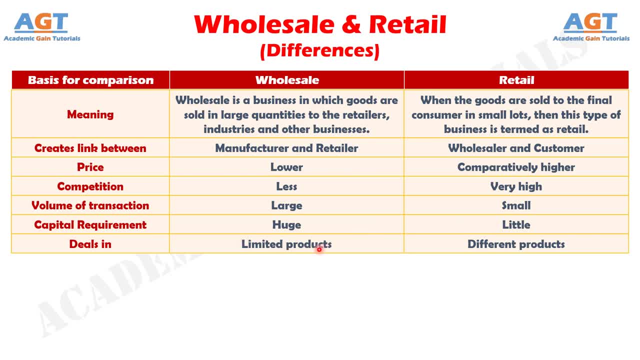 Number 7. Wholesale deals in limited products, whereas retail deals in different products. Number 8. Area of operation of wholesale is extended to various cities, whereas area of operation of retail is limited to a specific area. Number 9. Art of selling is not required in wholesale, whereas 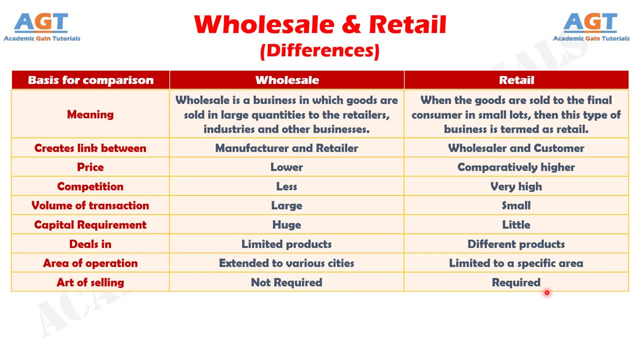 art of selling is limited to a specific area is required in retail and difference number 10. there is no requirement of advertising in wholesale but retail business requires advertising to grab the attention of customers.